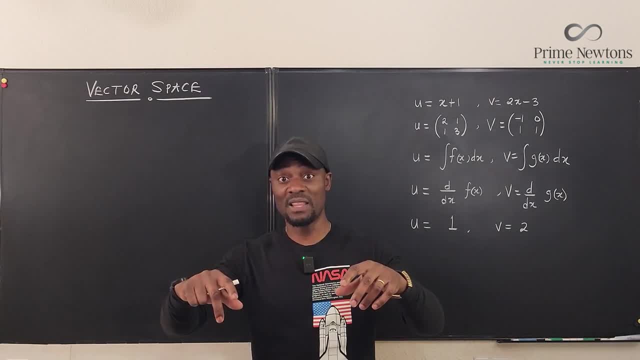 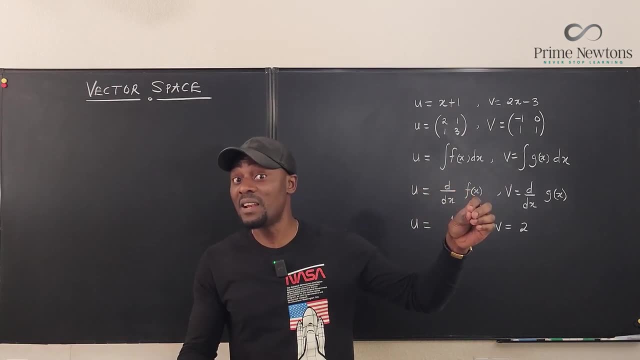 each other. that is, you can take one thing and add it to the other one in that set. and the second thing is you can stretch them by what we call scaling- it's called scalar multiplication- or you can compress them, you can make them bigger or smaller and you can add them to each other. those are the two things. 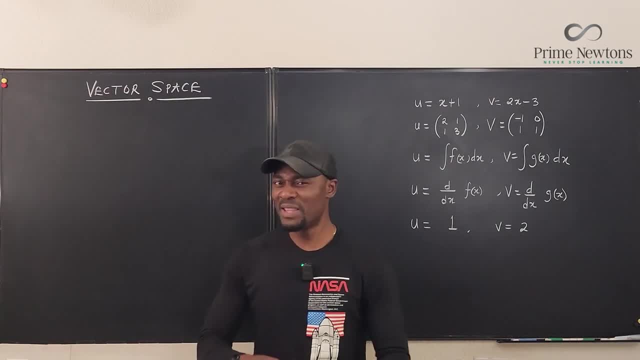 you need. so there is nothing else. just think of any set of stuff that you can add together such that when you add them together, the addition will still be behave as if it was in the set or the set of things that you can add to each other. 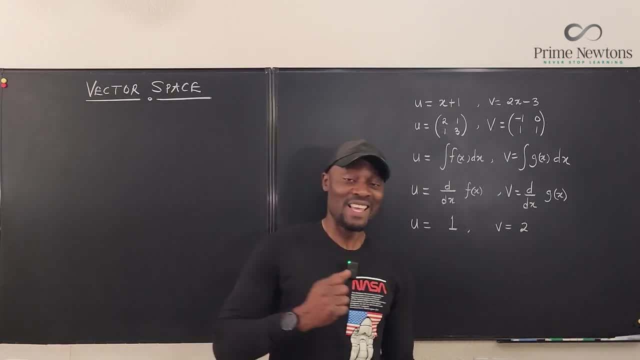 already right, okay. and the second thing is: if you pick anything in that set and you multiply it by a scalar quantity, a scalar quantity is- let's just for the sake of simplicity, let's just say- any real number. if you take any real number and you use it to multiply, let's not put zero now, because zero has a special 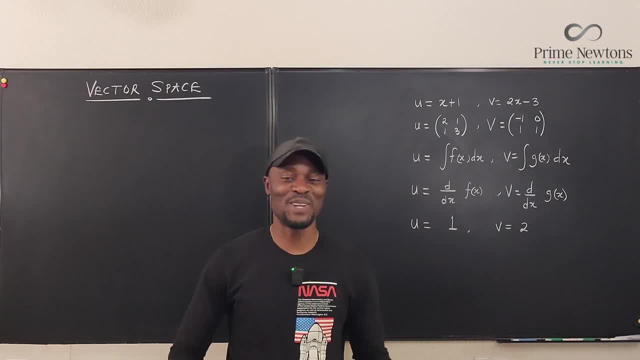 characteristics. zero makes everything disappear, so let's avoid zero. if you take a nonzero scalar and use it to multiply that thing, if it gets bigger or smaller, it's still. that thing is just a smaller version of it. so that's the idea of a vector space. so let me write the definition now. this: 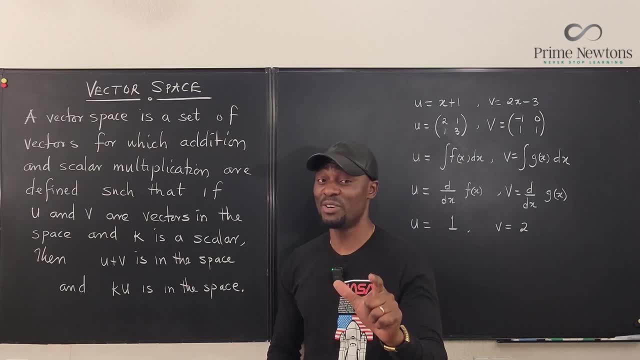 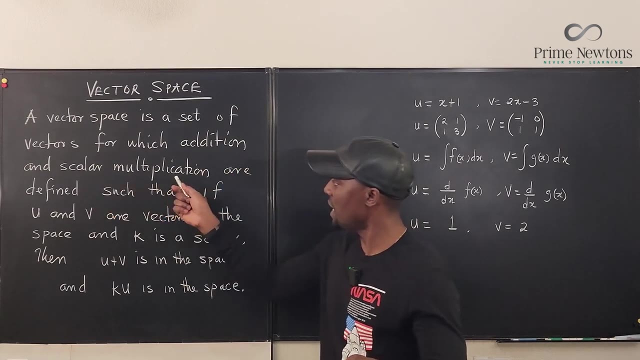 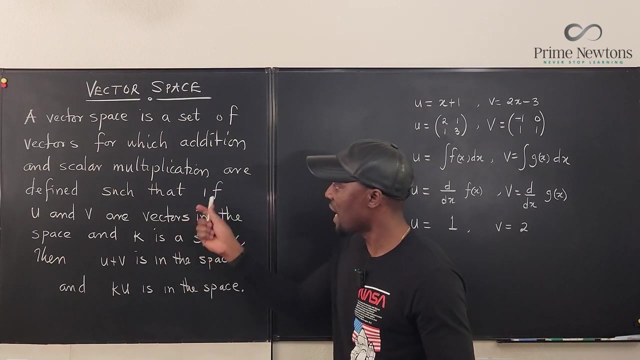 looks like a very long definition but it is necessary for you to have all of the most important concepts in the definition. it says a vector space is a set of vectors for which addition and scalar multiplication are defined. so you can perform addition and scalar multiplication such that if you have u, 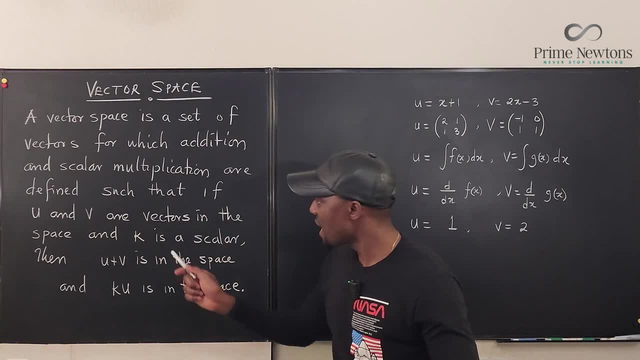 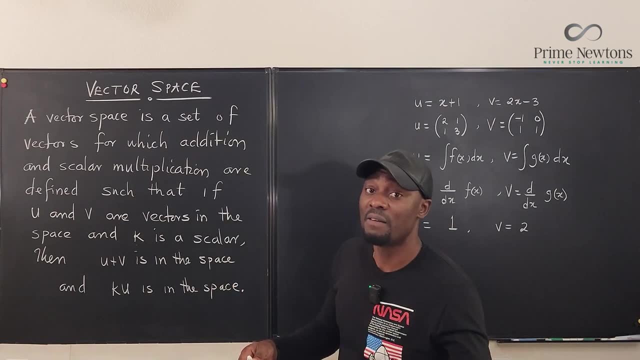 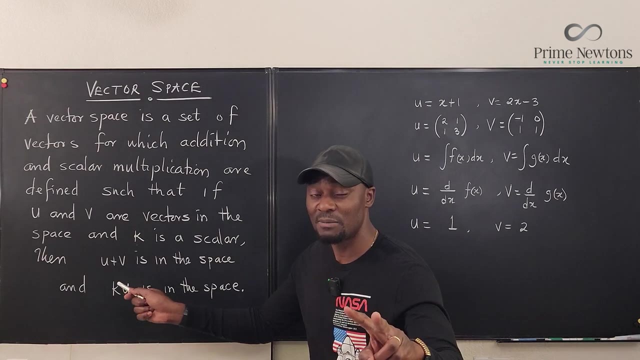 and v as vectors in that space and you have a certain k, which is a scalar quantity like one, two, three, four, one half minus seven, that's k. then whenever you add u and v, any two vectors in that space together, the new vector you get is also in that space. 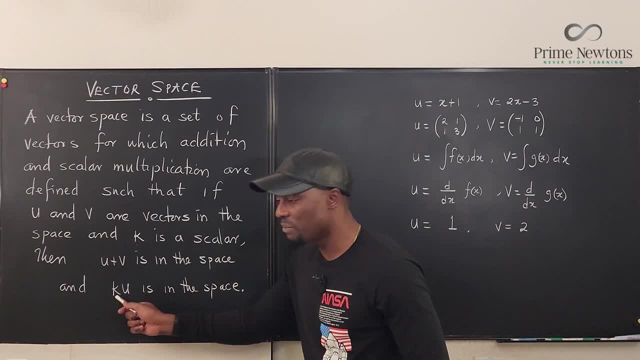 and the second point is: if you multiply a vector by a scalar, the new or the magnified or the contracted vector is also in that space. then you say that this is a vector space. however, there are some other things that the process that you just performed, whenever you add or whenever you multiply by a scalar, they 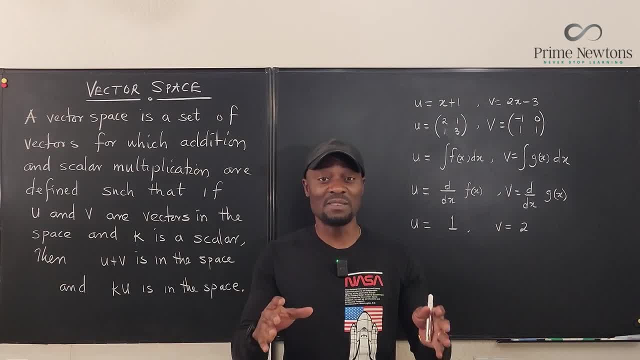 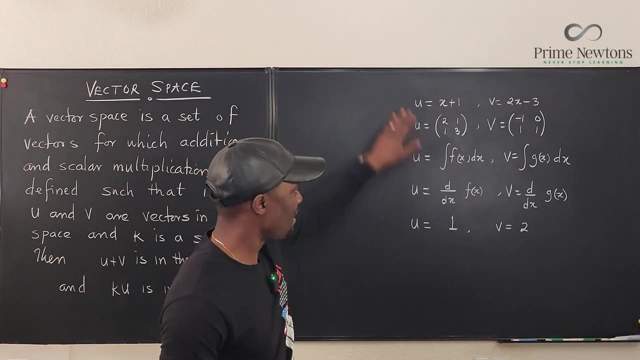 must have a certain behavior. those things that define their characteristics are what you call the axioms of a vector space. now, just to explain what I've just said, let's look at the examples that I have here. let's assume I have five examples of vector spaces. so let's say there's a vector space that contains 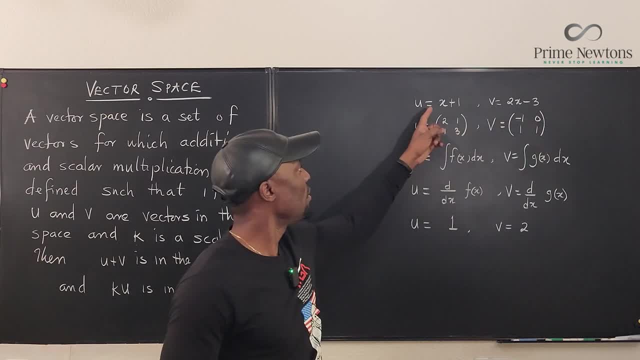 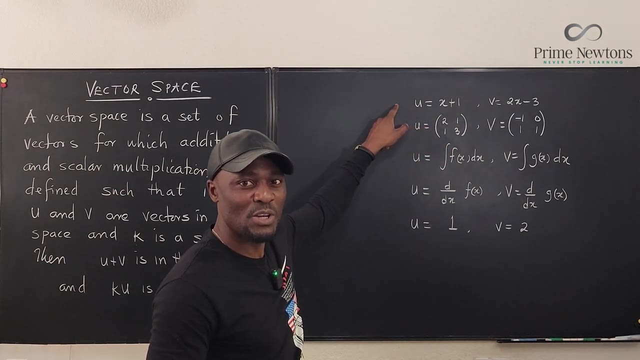 polynomials. these are polynomials. okay, a polynomial of first-degree. so this is X plus 1. this is also a polynomial of first-degree, first degree question. do you think you can add u to v? can you add them together? yes, if we add x. remember, this is the set of polynomials of first degree. if i add this to this, my answer: u plus v. 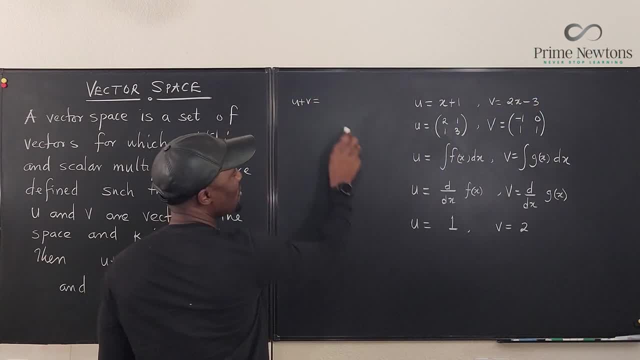 let me do it here. so i have u plus v is going to be. if i add this to this, what do i get? i'm going to get 3x minus 2. 3x minus 2. is this a polynomial of first degree? yes, therefore, it is the new. 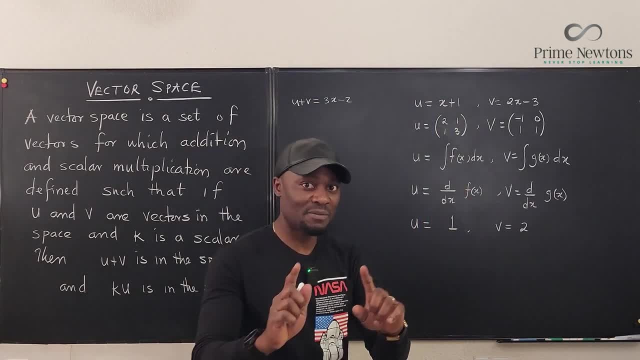 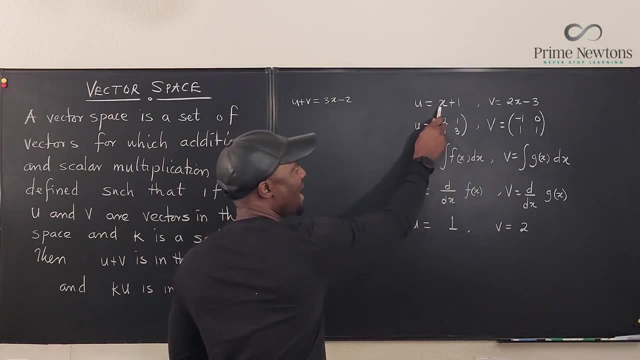 polynomial is also a polynomial of first degree. therefore it is in the vector space. second one: if i choose this and i multiply it by 5, 5 times, this is 5x plus 1. so you notice that 5 times x, 5u will be equal to 5x plus 5. 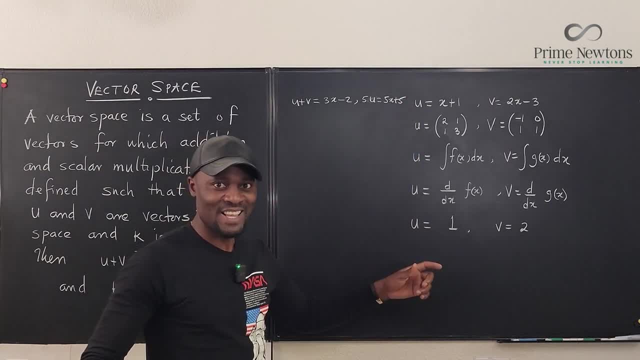 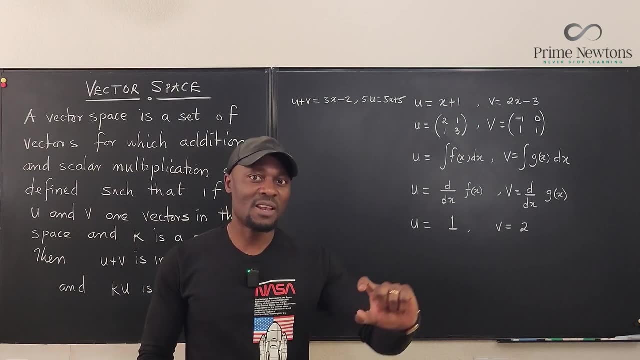 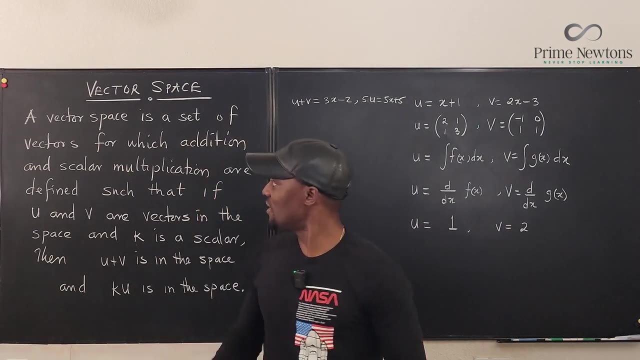 is this also a polynomial of first degree? yes, so that's the general idea of what a vector space is. addition and scalar multiplication are the most essential. there's some other properties we're going to talk about, but at least these are the beginning characteristics. there must be addition. 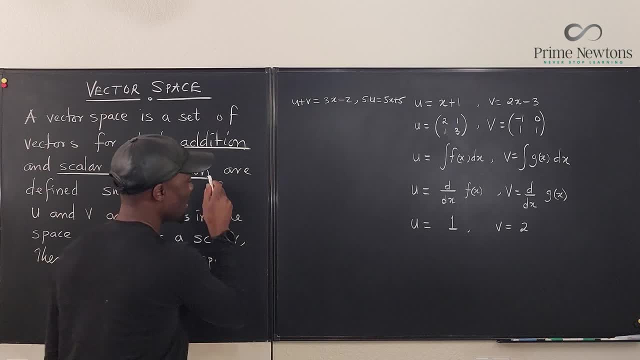 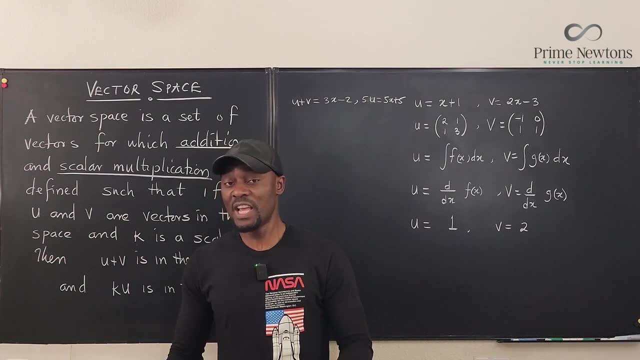 and there must be scalar multiplication. now some professors will say: these are axioms, which i think is a part of the definition of a vector space. so i'm going to talk about that in a little bit. it is, it is. it is described as the well-defined axioms- well-defined for addition and well-defined. 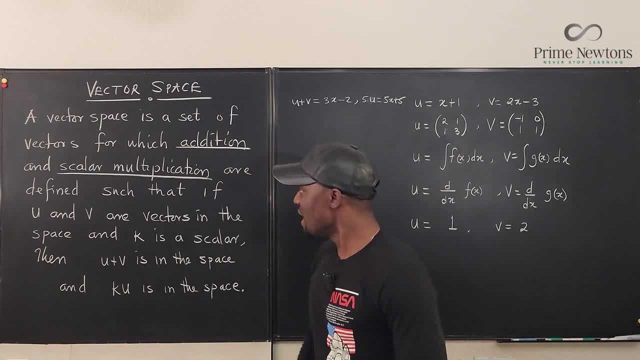 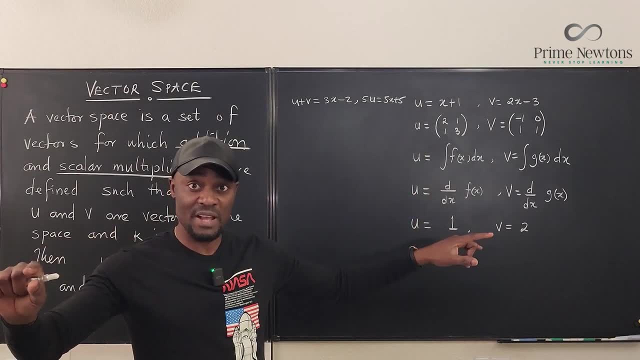 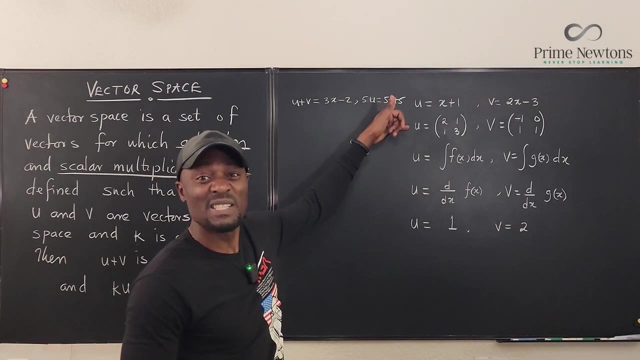 for scalar multiplication. okay, if you have this at the back of your mind, that applies to everything here. this is a. the real number line is a vector space. the, the, the euclidean plane, is a vector space. this is a vector space. if you have a set of two by two matrices, it's a vector space. why? 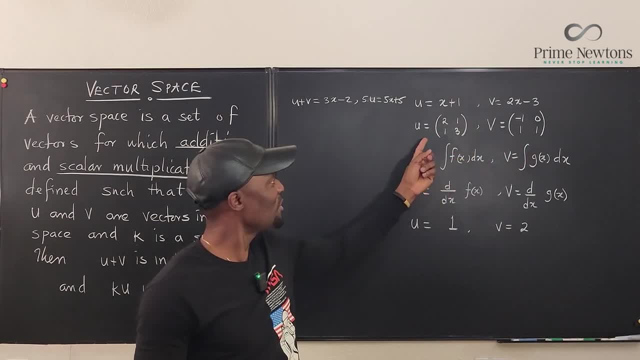 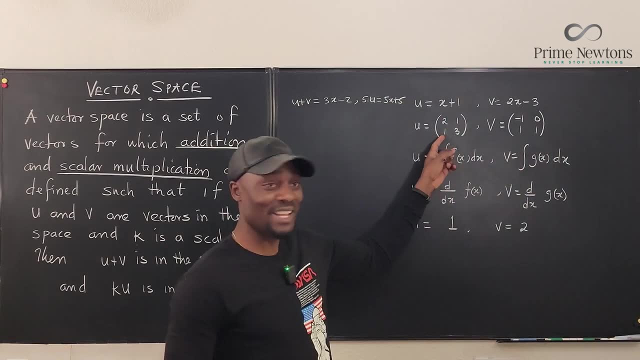 because you can multiply this by the number line and multiply this by the number line and multiply this by the number line. you can add these two together and you can multiply a matrix by a scalar, and if you add two matrices, you'll end up with another matrix that looks like this. so the 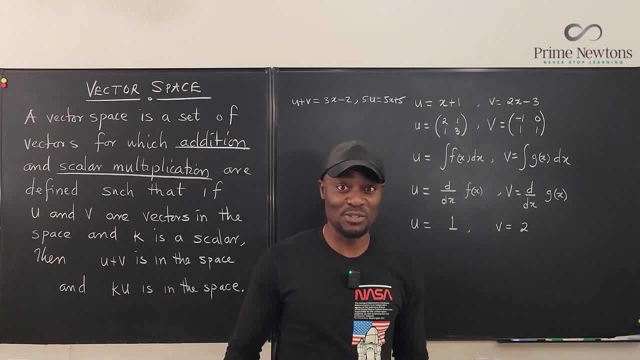 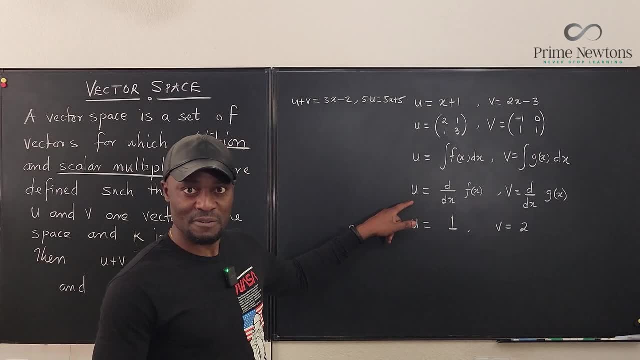 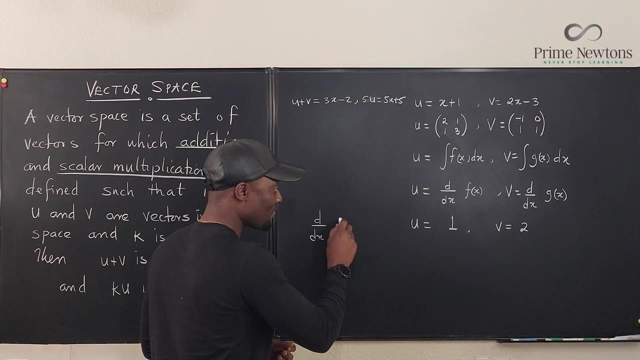 set of all two by two matrices will be a vector space because it satisfies these two conditions. okay, what else? derivatives? you can add derivatives, the derivative of the derivative, let's say ddx of sine x plus cosine x. you see, that is basically what. how do we get? this is the 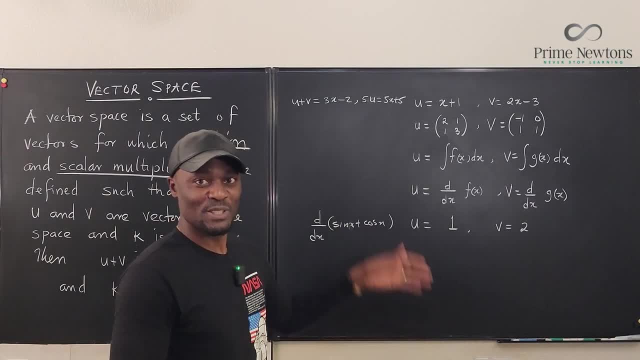 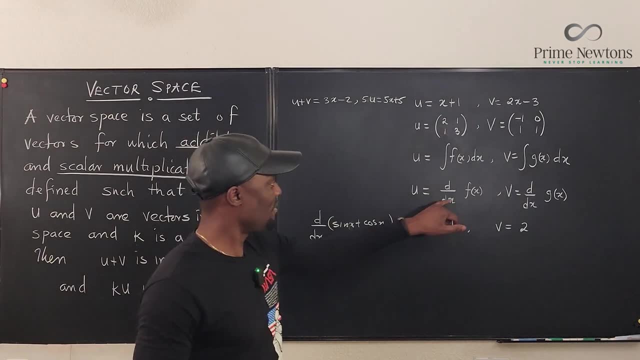 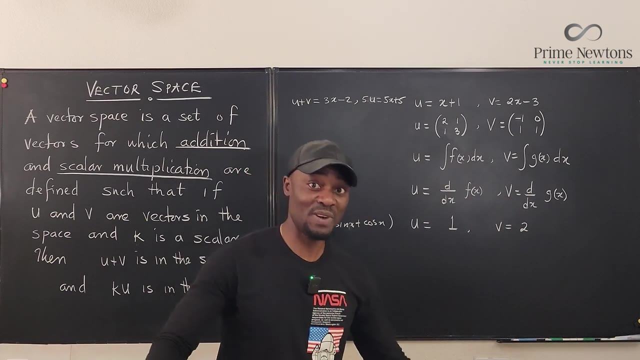 derivative of sine x plus the derivative of cosine x. so the derivative of all functions that are differentiable is just: you just pick a differentiable function. you can put: u plus v is just going to be ddx of f of x plus g of x. that's another function that is differentiable. 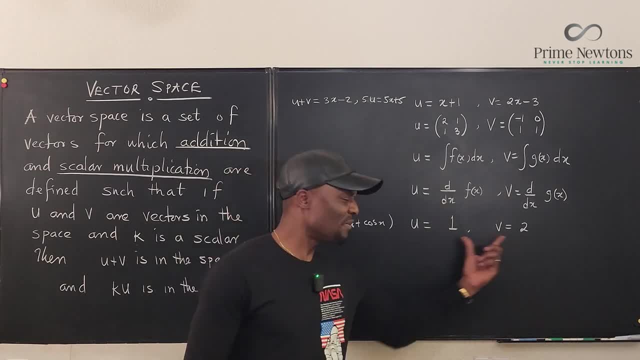 the same thing for functions that can be integrated. the same thing for just numbers, for just scalars, because you can add 1 to 2 and you can multiply this by 2 and whatever you get will always be a number. now the mystery of a vector space is is gone. so what are the axioms that you need to know? 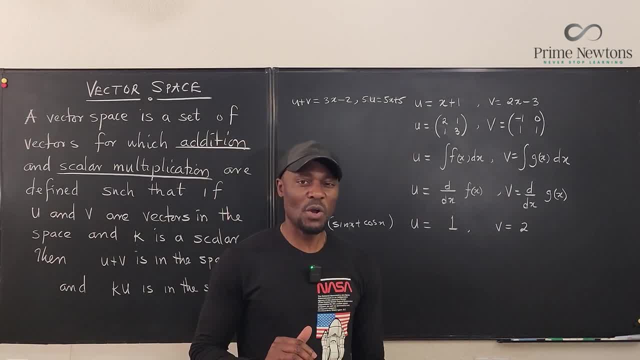 now. this is where students begin to struggle, because we're no longer used to memorizing things that we understand. you have to memorize every single axiom, maybe not in the same order as your neighbor will memorize it, but you have to know everything about the axioms of a vector space. 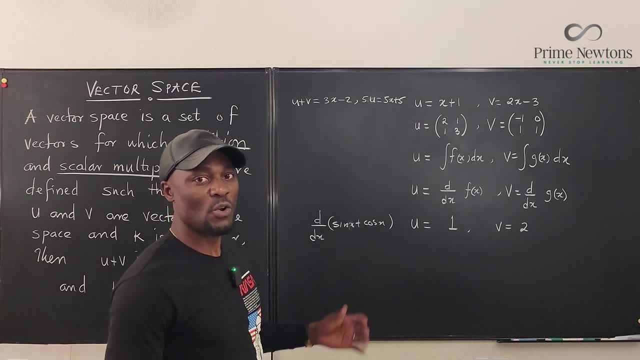 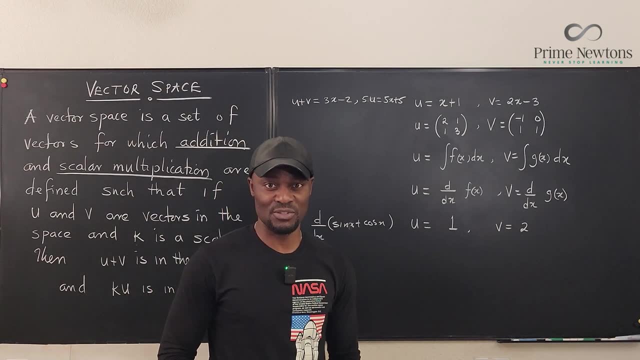 So I'm going to erase this and list them out, And all you have to do is make sure you remember them and you can perform them anytime you're asked to verify the axioms of a vector space, Let's do it. So let's just run through the axioms. 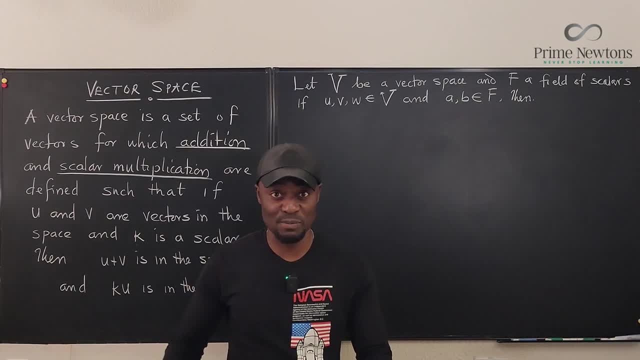 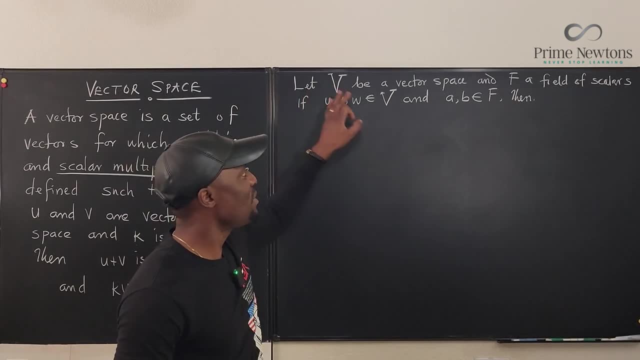 And you have to be able to show that this is true for any vector space that you are given. Okay, number one, let's look at the details. Let V be a vector space and let F be a field of scalars. okay, 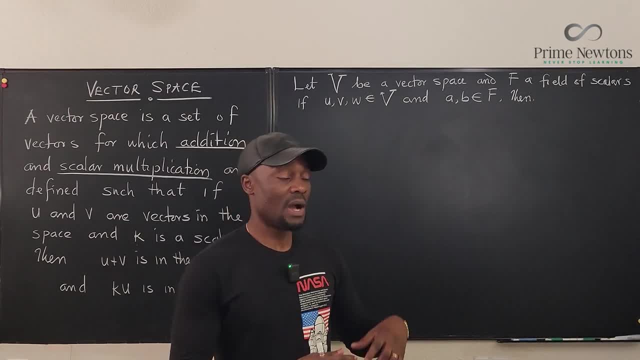 Now my examples so far have been on real numbers. I've used 1,, 2, minus 7, all that. Those are real numbers. Sometimes the field of scalars is complex numbers or imaginary numbers. So just know that we're dealing with scalars. 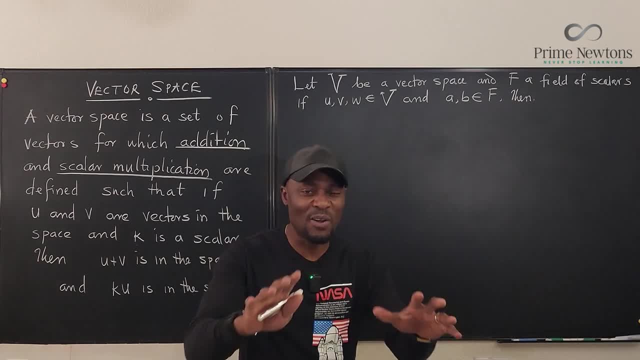 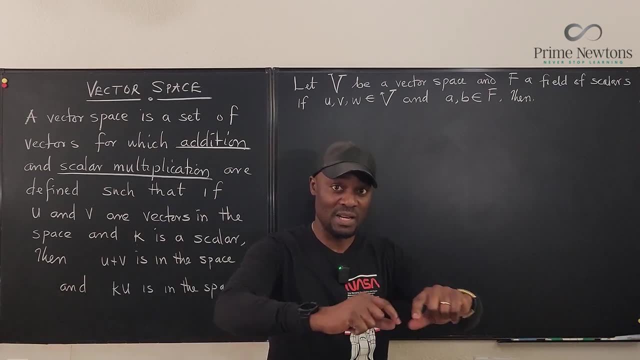 That's why we use the word scalars, because sometimes it's not real. But for now, let's just talk about real numbers, okay. So what I say? The field of scalars, I'm talking about real numbers on the number line, okay. 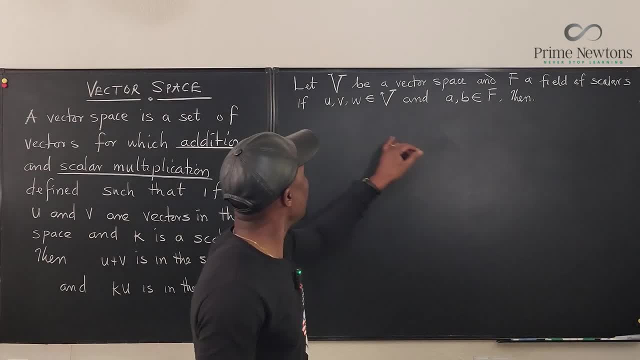 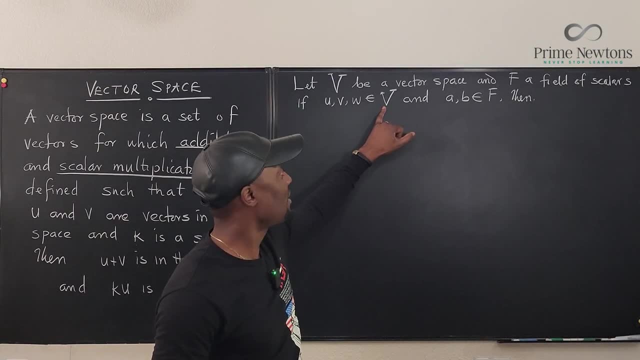 They don't have to be rational, They just have to be real. And if U, V and W, these are vectors in V, in the vector space, and A, B are scalars in that field, then the following will be: all the eight things I'm about to say will be true. 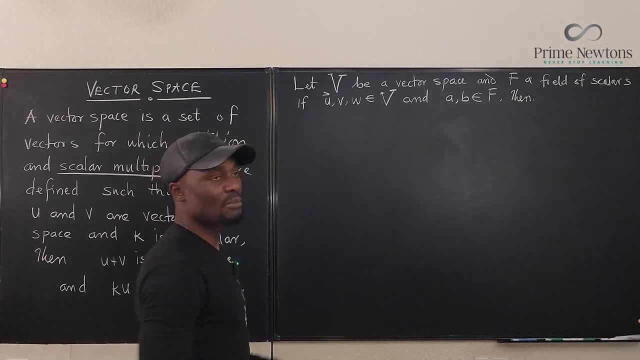 Some professors want you to do this. okay, I'm not going to do that arrow thing. Okay, If a professor wants it, you have to do what they want. But right now I'm just going to start with the very first one. 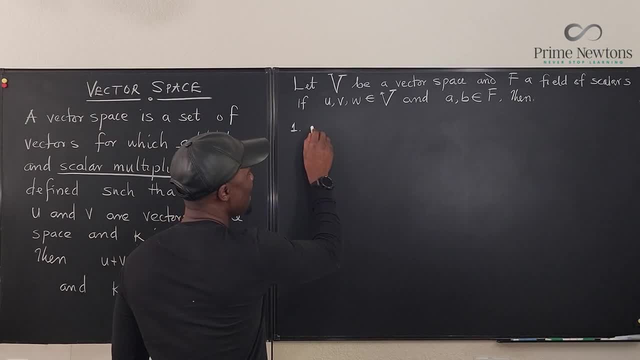 The very first one is that U plus V, axiom 1, U plus V is equal to V plus U. This is the commutative property. of addition, Everybody knows that 1 plus 2 is equal to 2 plus 1.. 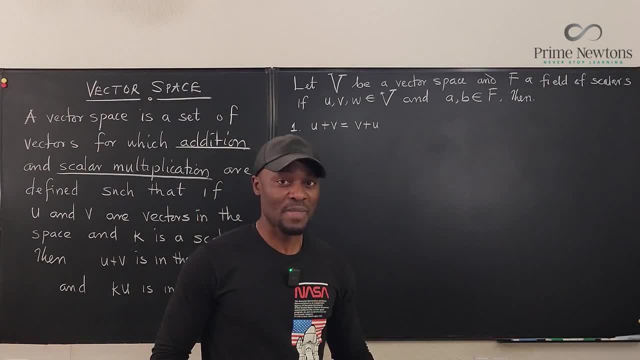 And that has to be true for any vector space. So whether you're adding a polynomial and you switch the orders- adding polynomials and you switch the order- it doesn't matter. You should still get the same answer, right? Okay, so that's what this one is all about. 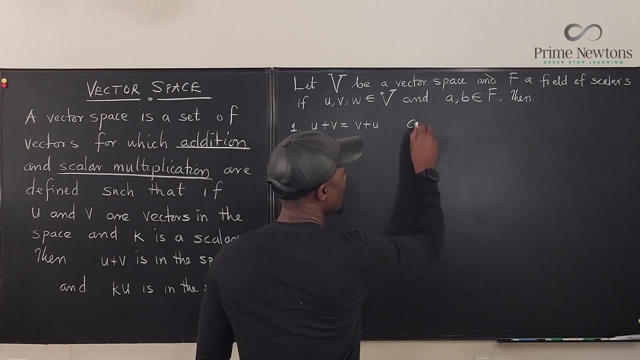 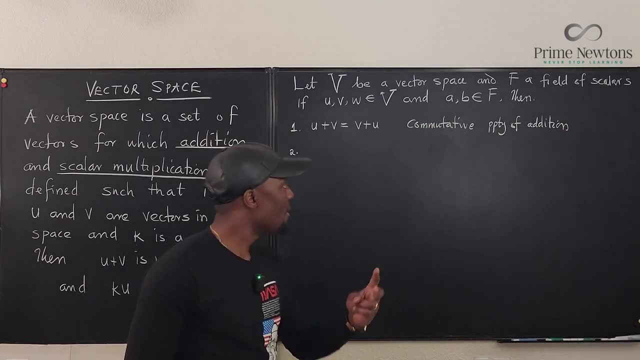 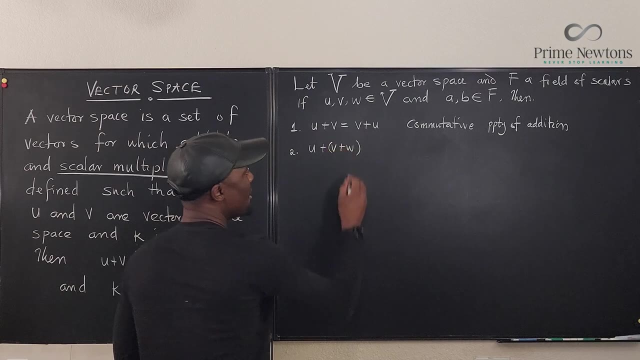 Number two. So this is what you call the commutative property of addition. The second thing you need to know is that when you are adding, you can say U plus V plus W, but you can add the first two before you add the third one. 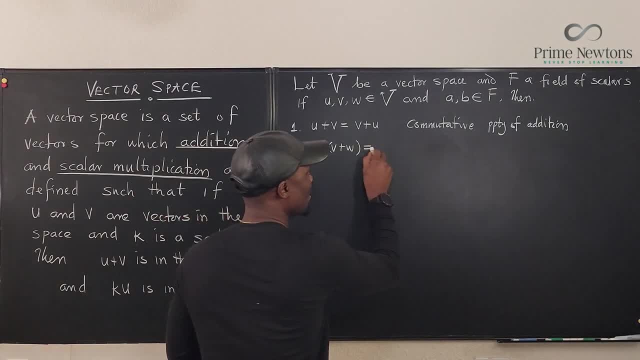 It doesn't matter the order in which you add, So you can have U plus V plus W. It is important that you have this also memorized. And this is the associative property. Okay, I'm just going to write that short version like that. 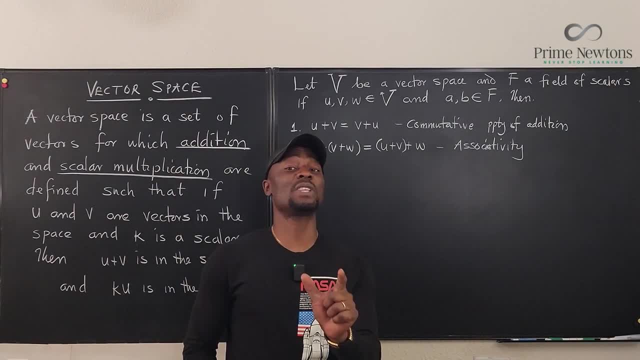 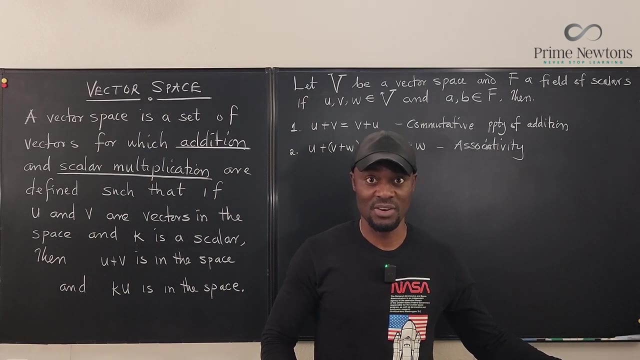 The third one is very essential. You need it almost every time, And it is the existence of the zero vector. There has to be some vector in that vector space Such that when you add that vector to any vector it does not change the other vector, right? 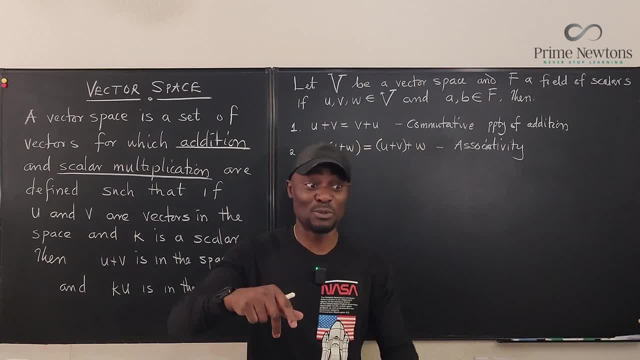 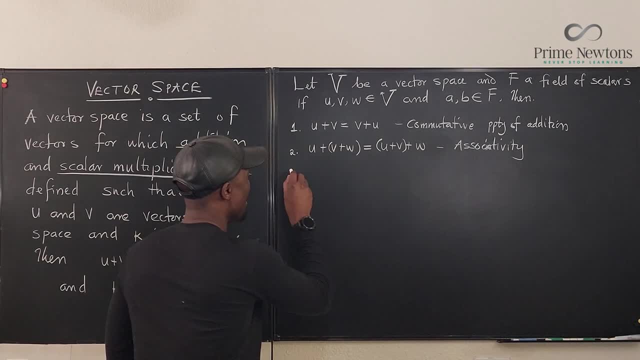 Just as when you're dealing with numbers, when you add zero to something else, something else doesn't change. Zero plus five is always five. So number three is: there is a zero vector which is denoted this way: Okay, such that zero plus U is equal to U plus zero. 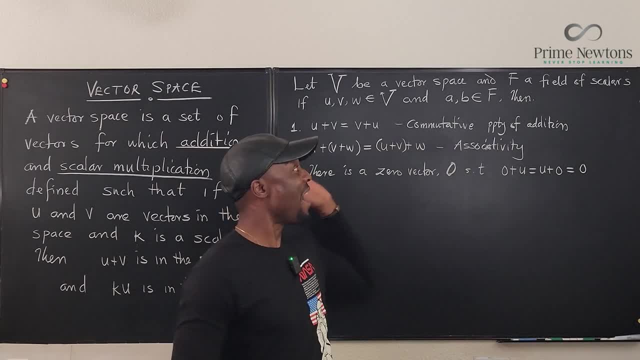 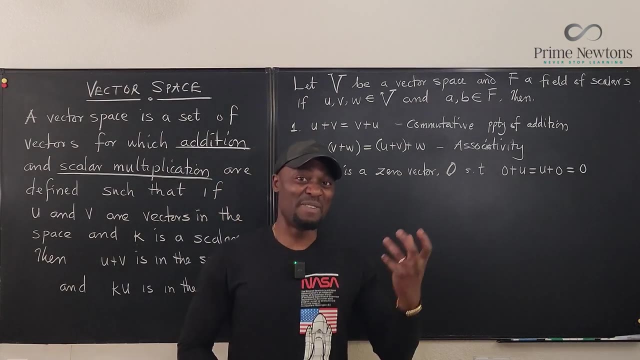 And it's equal to zero for all U, for every U, that you see every vector. this is always true. Now, that is the zero vector. Okay, number four. Number four says every vector in the vector space has another guy. 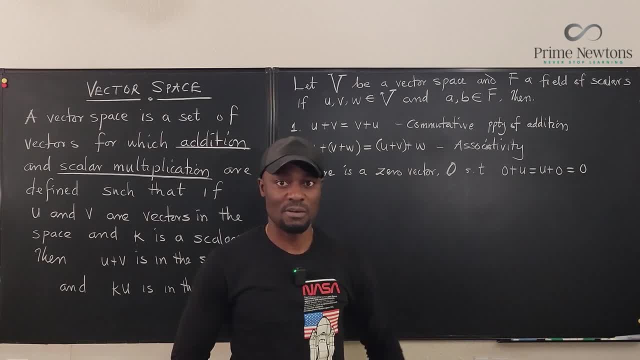 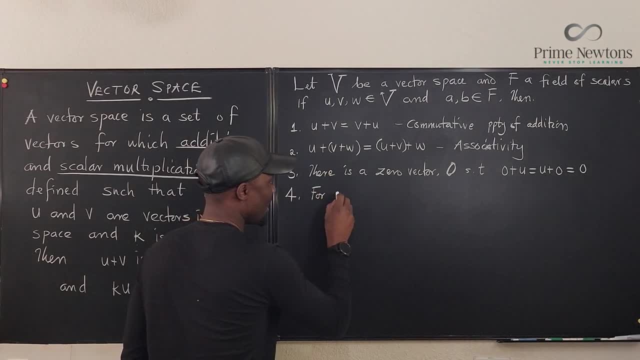 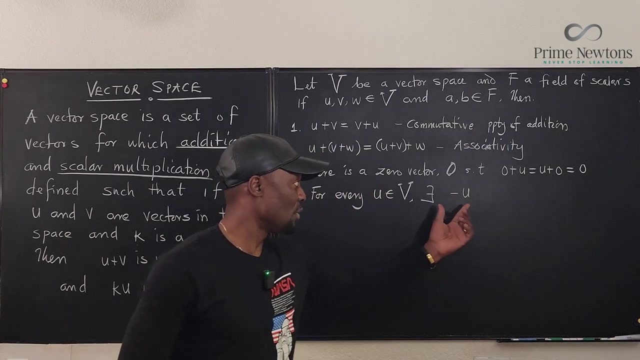 Such that when you combine the two of them, it could give you zero, And that's what you call the additive inverse. Okay, for every U in the vector space there exists a negative U. Okay, now some people use a negative U. 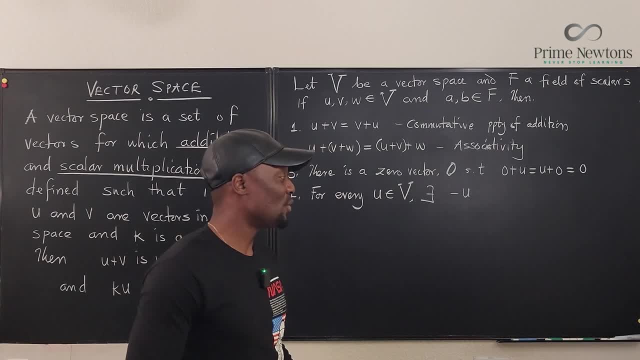 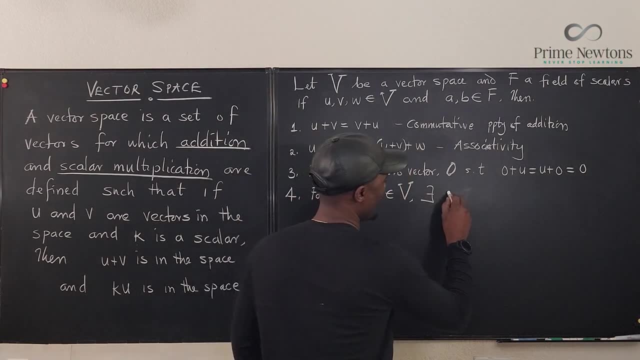 some people say it's a Y. Okay, Now maybe I should use U prime. It doesn't matter how you symbolize it. Let's say: for every U there is a, let's call it U prime, such that U plus U prime is equal to zero. 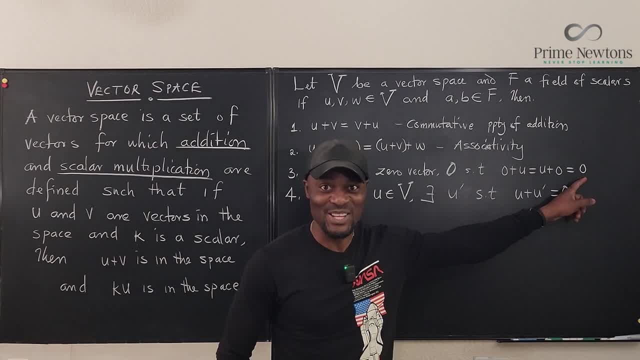 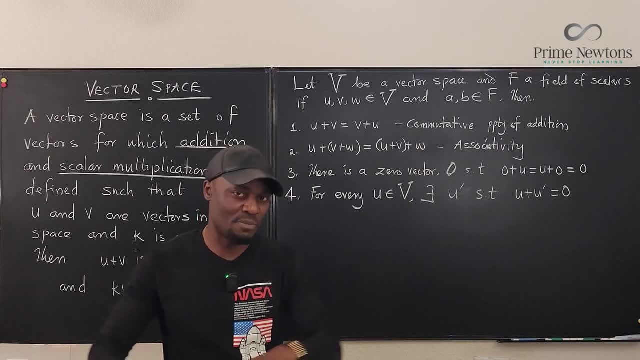 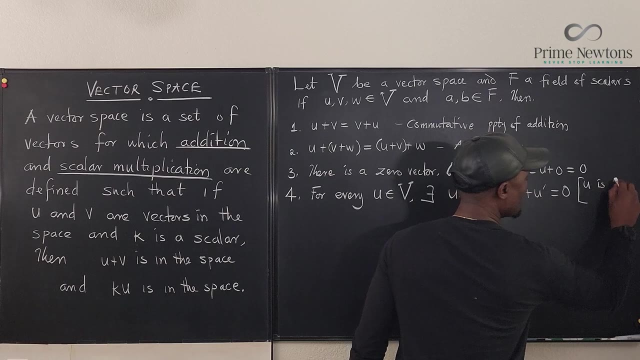 is equal to the zero vector. Okay, so there has to be a U. This is what you call the additive inverse. It is what you must add to something to make it a zero. So let's write something here. So U is the additive inverse. 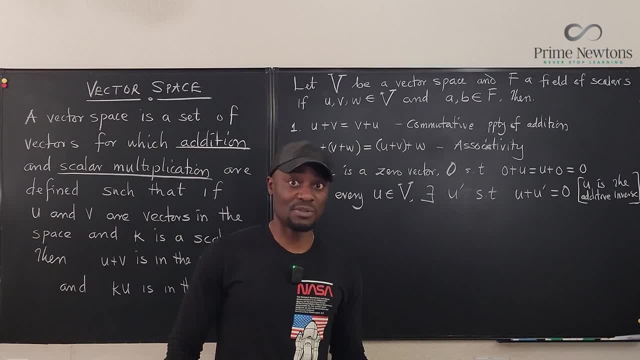 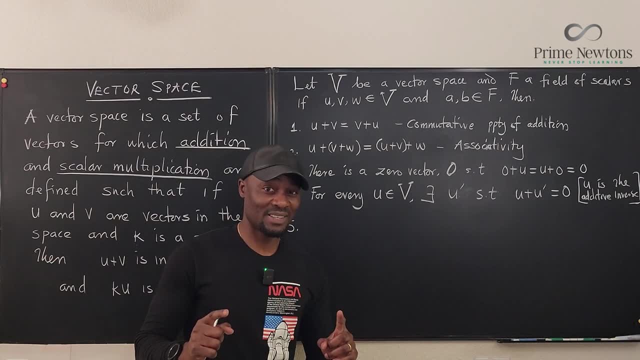 Okay, just as minus five is the additive inverse of five. When you add minus five to five, you get zero, right? Okay, number five. If you notice, all the things I've talked about for the first four have been about addition. 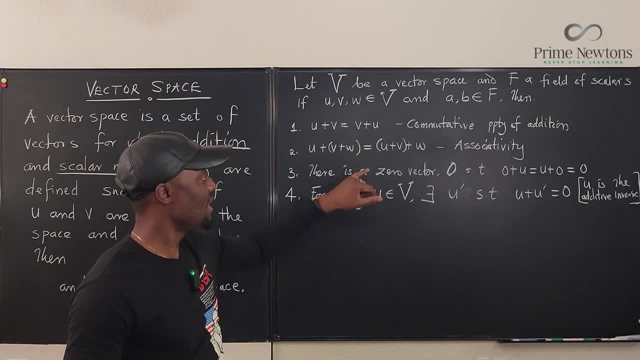 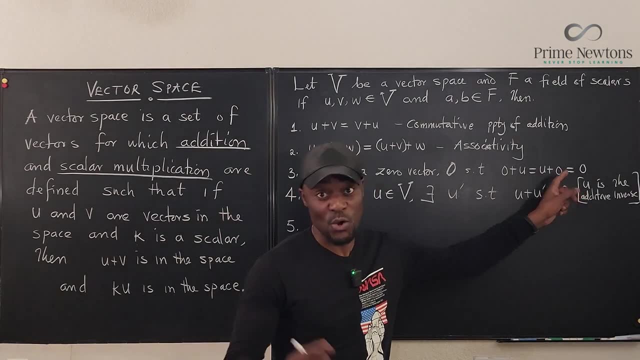 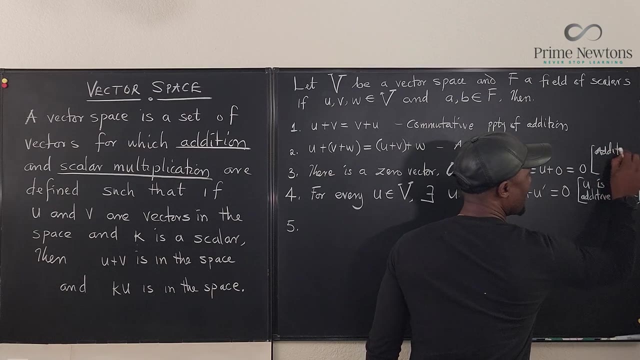 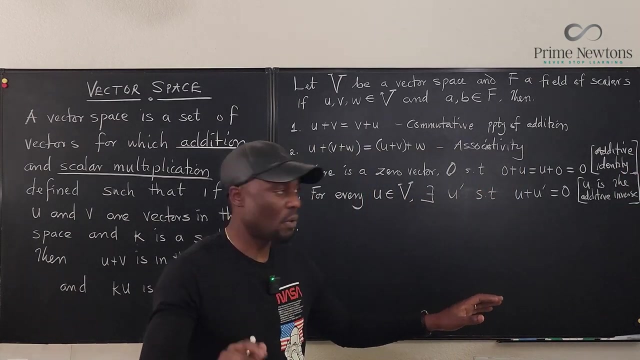 Commutativity of addition, associativity of addition, the existence of the zero vector, that is, the additive identity. Oh, I didn't even say it. This is the additive identity. okay, Additive identity. So it's easy for you to recall all four. 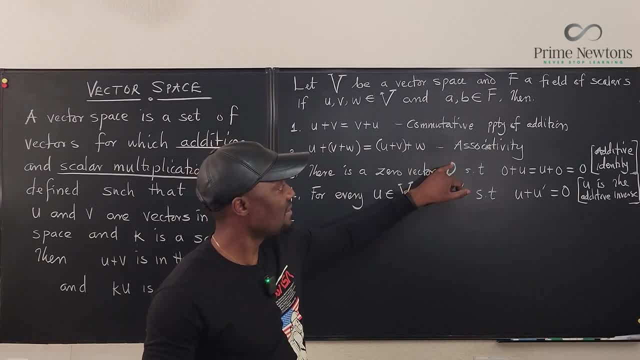 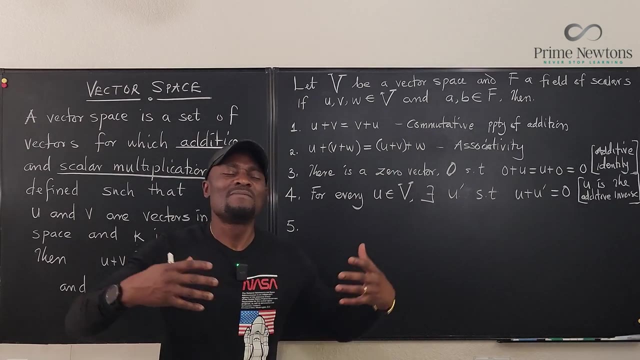 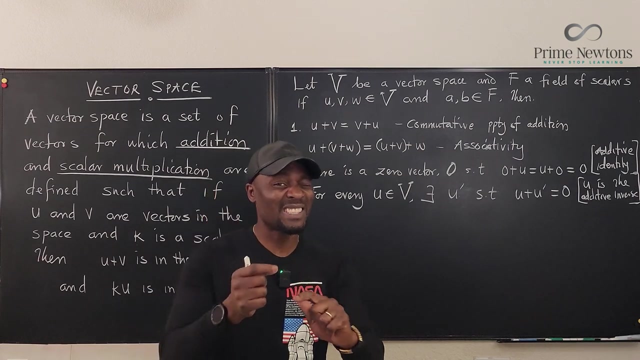 Commutativity of addition, associativity of addition, additive identity and additive identity: Okay, additive inverse, remember those four? number five now switches to multiplication. okay, multiplication says that there has to be, there has to be some multiplicative identity, and you know what it is. what is that thing? you will use that scalar that you will use to multiply. 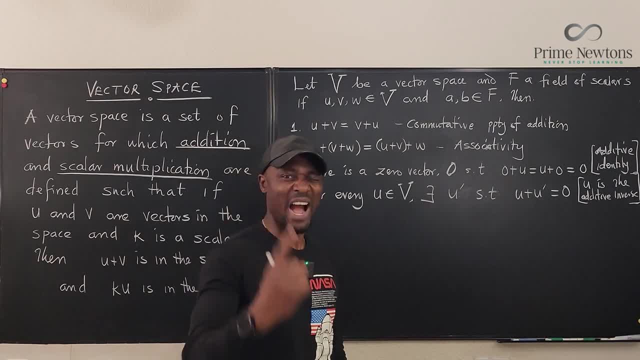 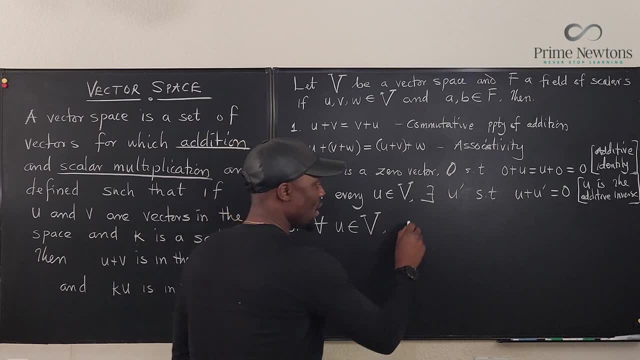 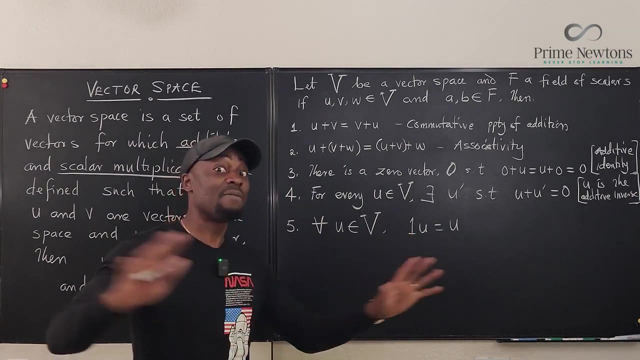 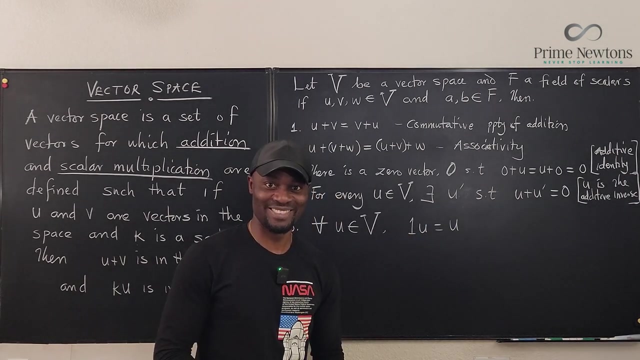 something and it doesn't change that thing. it's the guy called one. okay. so we say, for all u in the vector space, we know that one times u is equal to u, this one exists. every, every there has to be this guy. this guy is always there. okay, so one times u is u, it doesn't. 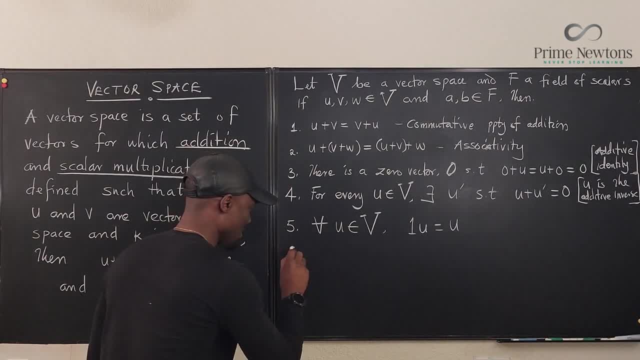 change anything. so let's go to number six. what does number six say? number six says a? a? u multiplied by a? u. sorry, let's change this to b? u. if you remember, a and b are scalars from our definition. so if you take a number two and then you use it to multiply three, 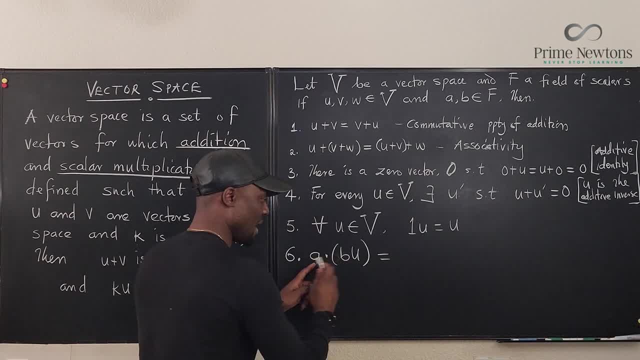 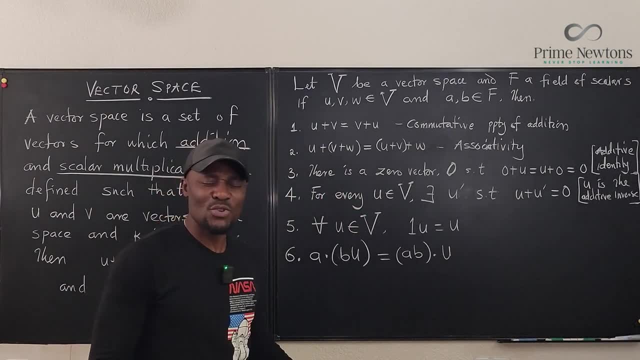 u. it's the same thing as multiplying the scalars: first it is a, b multiplied by u now. so you're going to say this is common sense. well, you have to be able to show it. sometimes it is not obvious, and sometimes it is the only way out of what it, whatever.